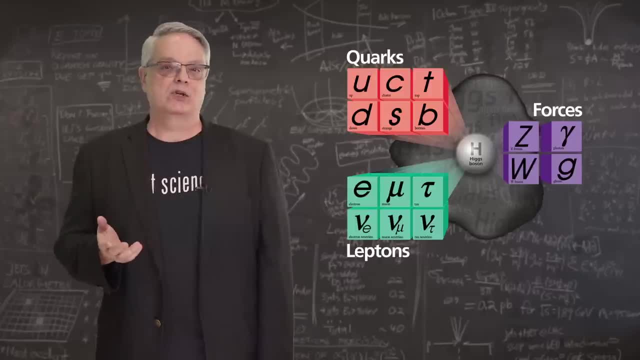 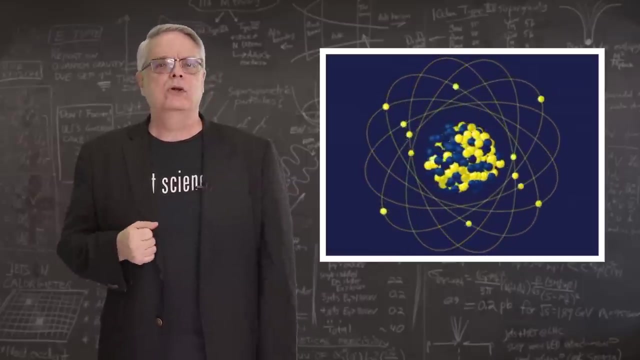 Because those particles decay, they don't stick around very long and consequently have very little to do with the familiar world around us. However, not all particles are unstable. The proton, neutron and electron of the atom are well-known inhabitants of the world we experience. We know that neutrons can decay under the right. 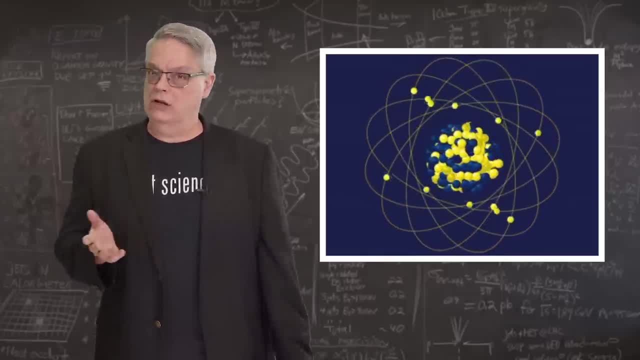 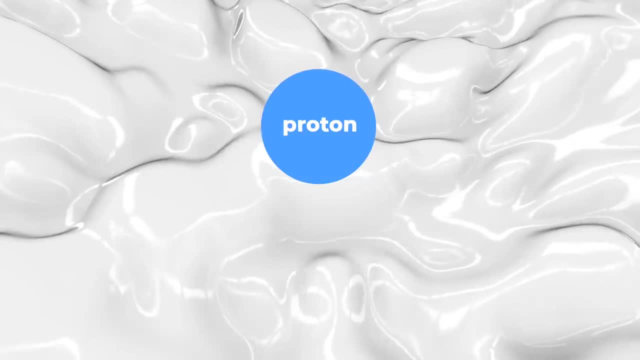 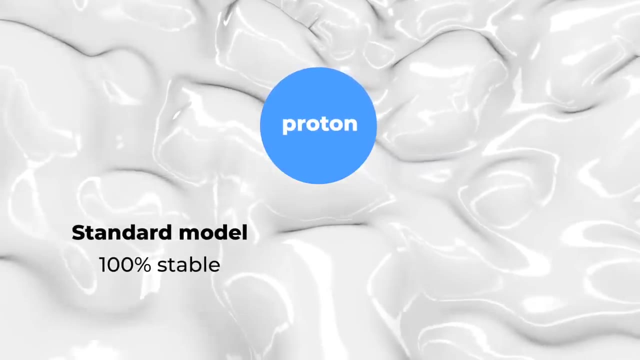 circumstances, so we can ignore them in any conversation about long-term stability. But the proton is a much more interesting particle to consider. It's because of two things. First, our best theory says that protons are 100% stable, meaning that they won't decay. By the way, the name for that theory is the Standard Model. 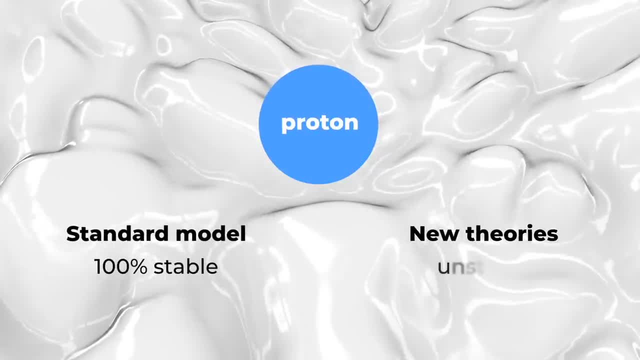 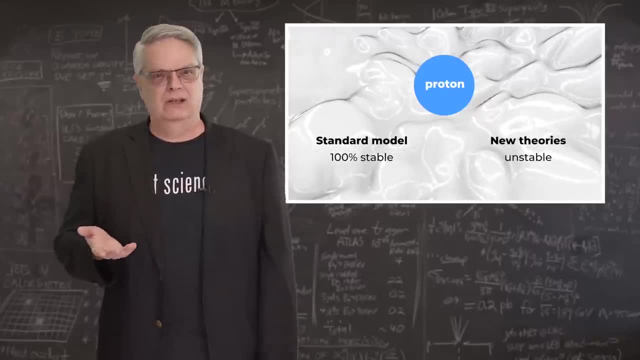 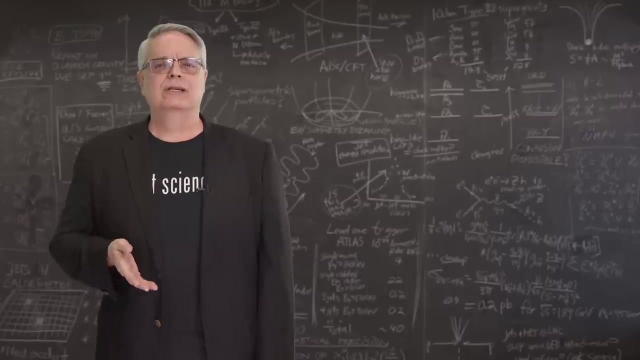 On the other hand, other theories predict that protons will decay, at least eventually. Some scientists hope these new theories will replace the Standard Model. so it's important to look for proton decay to see if these new ideas are on track. So first let's see why the Standard Model claims that protons are stable. 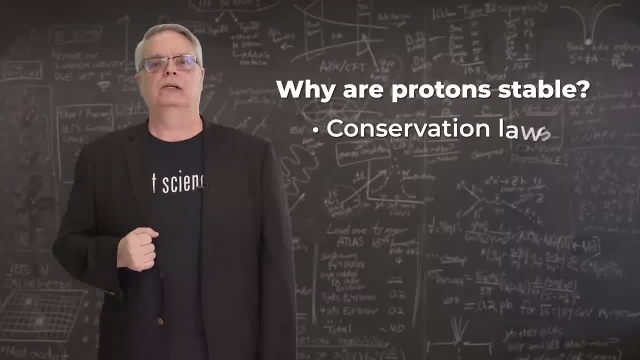 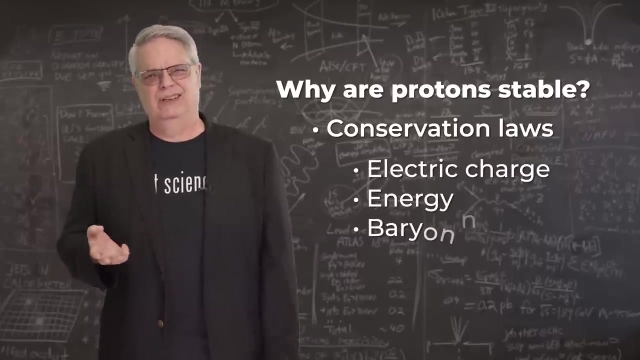 It all comes down to things called conservation laws. Conservation laws state that there are some properties that never change, no matter what. Three specific conservation laws are important in talking about proton, decay, Electric charge, energy and a more obscure quantity called baryon number. 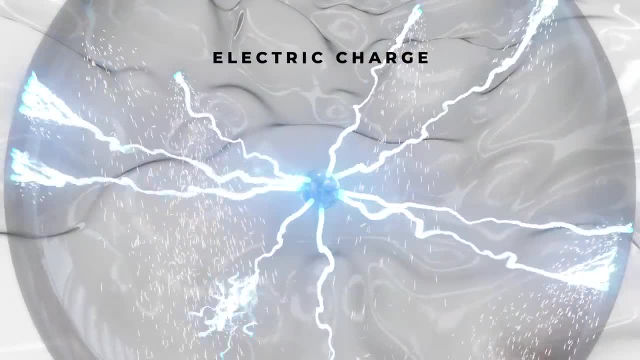 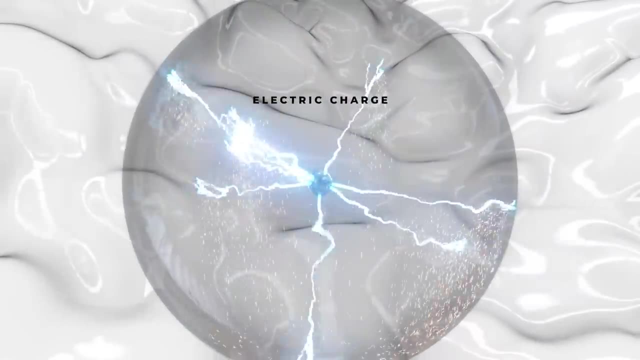 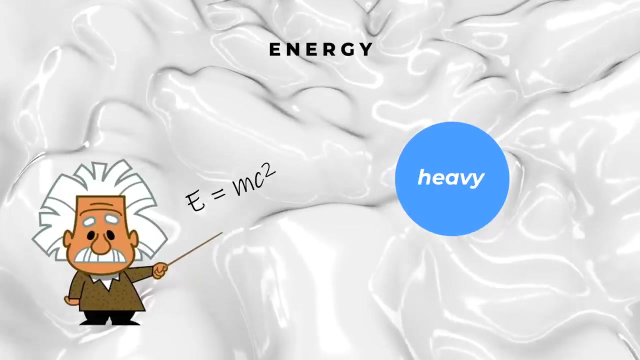 Electric charge is pretty familiar. Conservation of charge simply means that after the decay the amount of electric charge decreases. charge must be the same as it was before the decay. Conservation of energy has a number of implications, but the key one is tied to Einstein's equation. 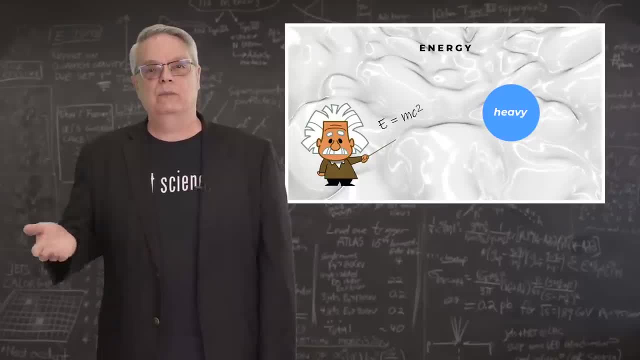 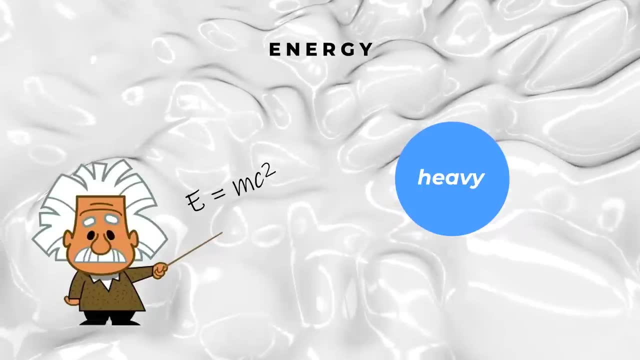 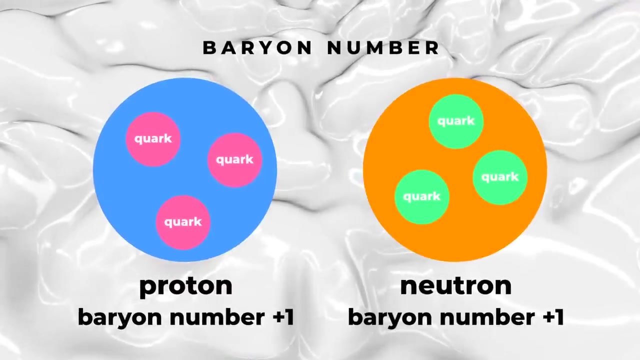 E equals mc squared, which says that energy and mass are basically the same For particle decay. energy conservation just implies that particles can only decay into lighter particles. Baryon number is much less familiar. Baryons are particles consisting of three quarks. 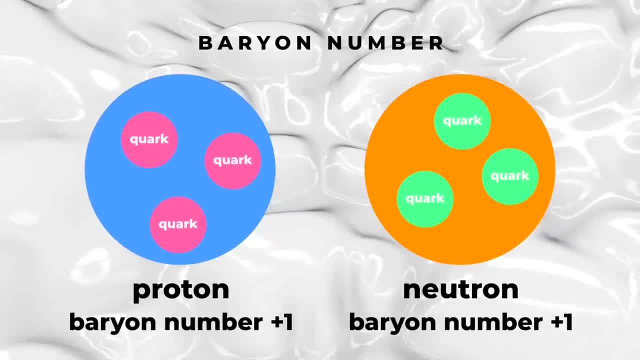 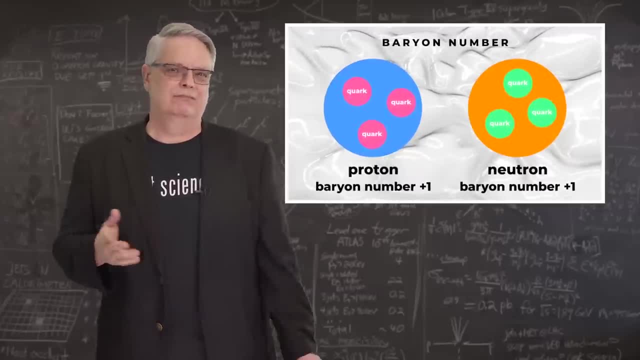 Quarks are one of the smallest known building blocks of matter, and protons and neutrons each contain three quarks each. Thus protons and neutrons are both baryons, but there are many kinds of baryons. Baryon number is simple. 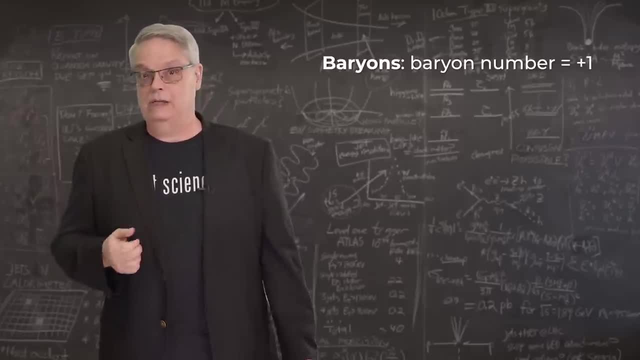 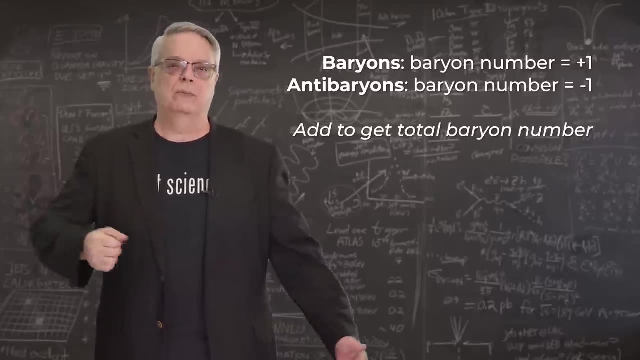 Every baryon has a baryon number of plus one. Antimatter baryons have a baryon number of minus one And to find the total baryon number you just add them up. For instance, at the LHC, when you smash two protons, each with a baryon number of plus. 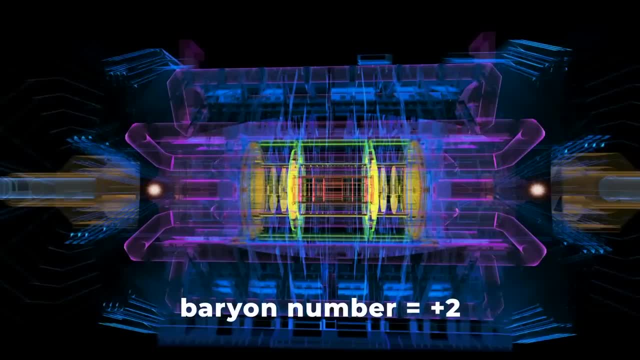 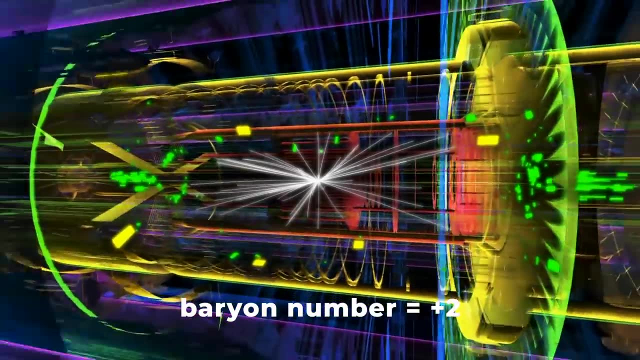 one, the collision has a baryon number of plus two. After the collision, no matter how messy and complicated, the baryon number is still plus two. So there have to be two baryons wandering around somewhere in the debris. 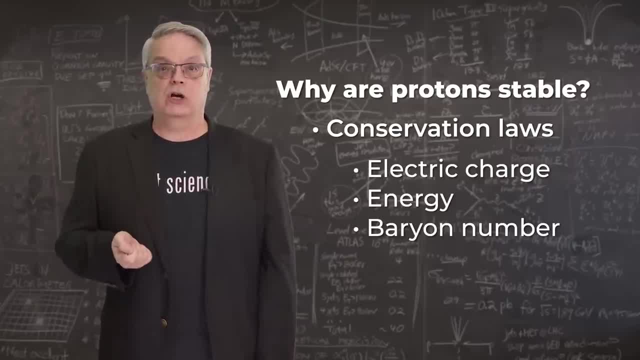 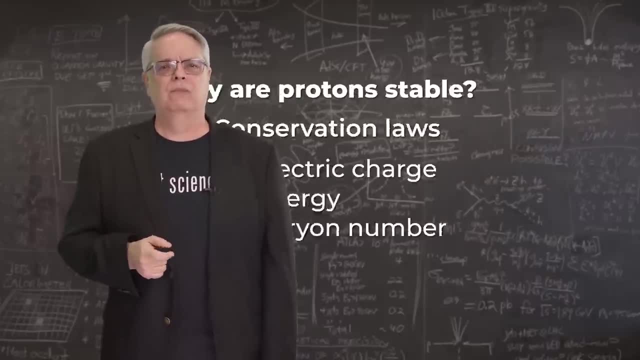 According to the standard model baryon number, electric charge is equal to the number of neutrons. Electric charge and energy are all conserved. There are many more conserved quantities, but let's just focus on these three. Let me give you an example. 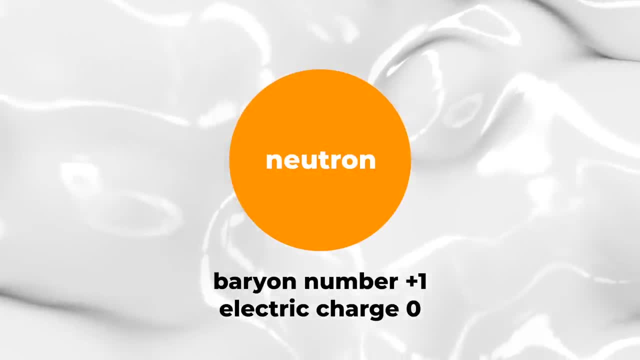 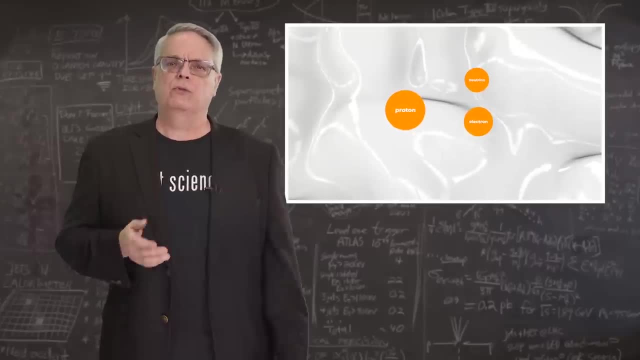 In the case of neutron decay, what happens is the neutron turns into a proton, an electron, and an electron antimatter, neutrino. Since both proton and neutron have baryon number of plus one baryon number is conserved in the decay. 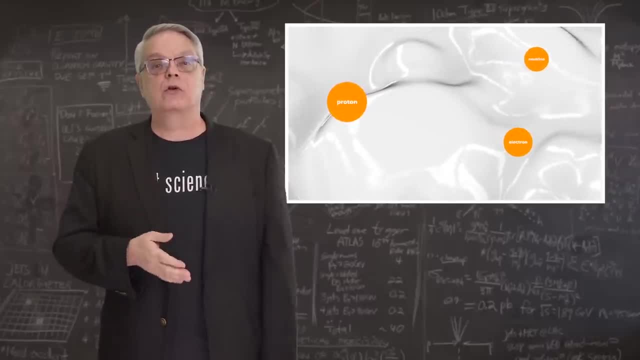 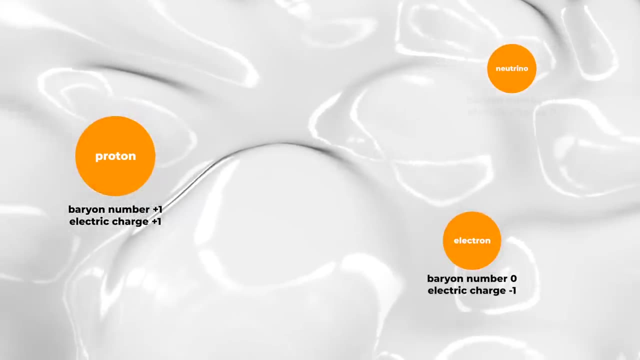 Plus one before and one after, Since the neutron has zero charge, the proton has plus one charge, the electron has negative one and the antineutrino has zero. we see, electric charge is conserved. It's zero before and zero after. 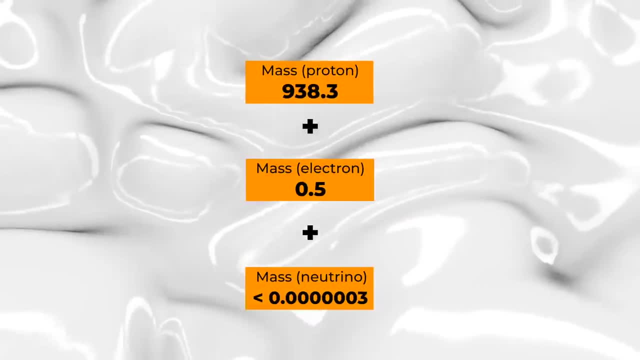 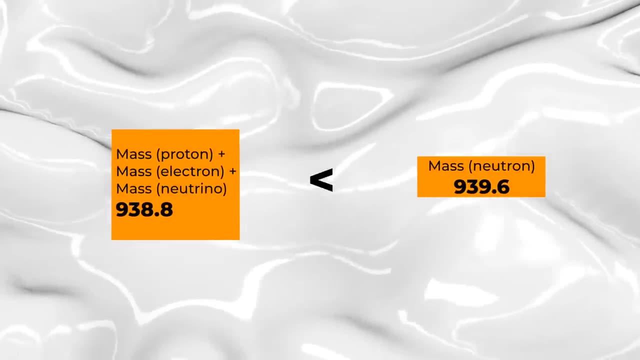 And on the energy front, when we add up the mass of the proton, electron and antimatter neutrino, they all have a total mass less than the neutron. That means neutron decay can proceed. as far as these three conservation laws go, The electron decay is conserved. 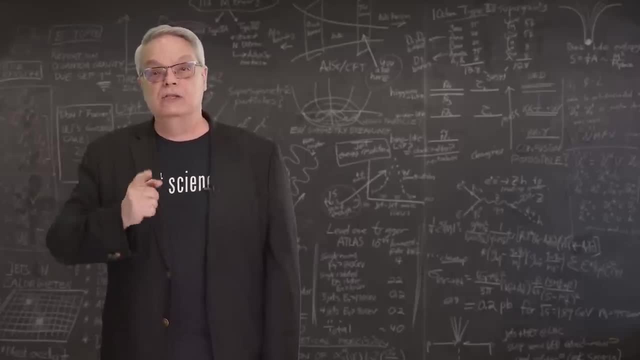 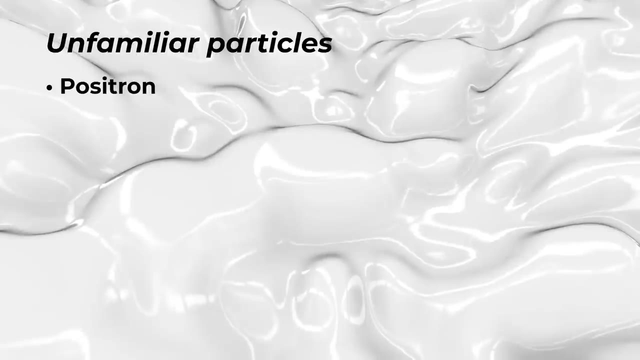 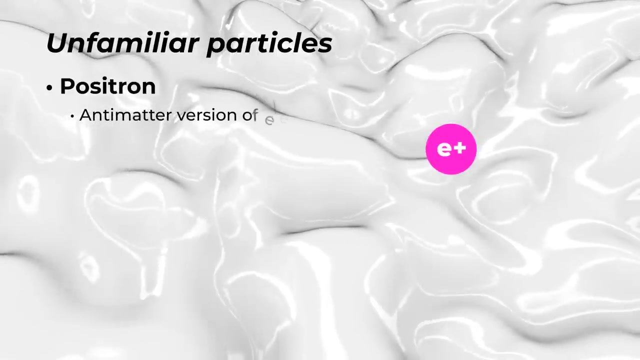 The neutron decay is conserved. Now let's think about proton decay. To do that, we need to introduce two particles that are well known to particle physicists but are not common knowledge. The first is called the positron. The positron is the antimatter equivalent of the electron, and the positron has plus. 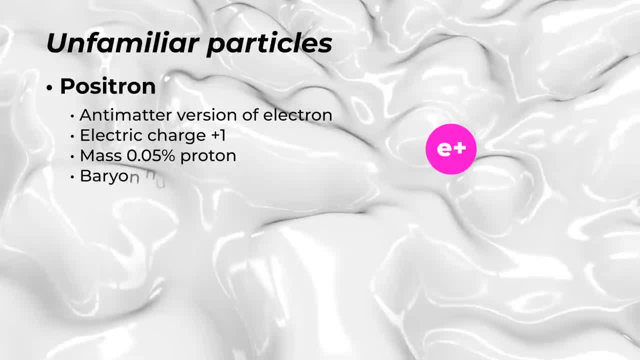 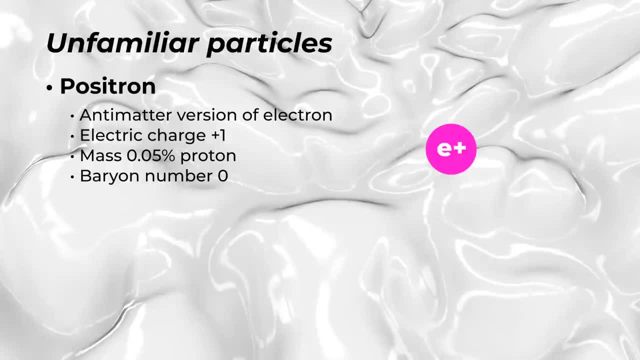 one charge. just like the proton, The positron is also much lighter than the proton, like 0.05% the mass of the proton. Because the positron isn't a proton, the electron decay is conserved. The positron isn't a baryon. it has a baryon number of zero. 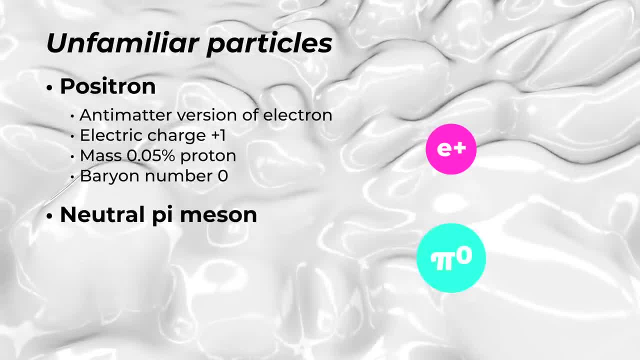 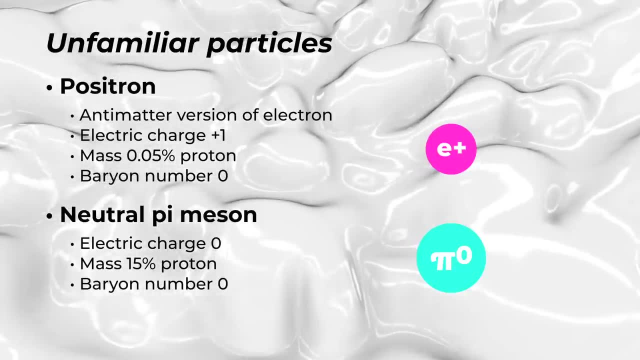 The second is called a pi-maison. It is also pretty light, with a mass of about 15% that of a proton, And it's not a baryon either, so it has a baryon number of zero. Finally, there's one more fact that's important, which is that the proton is the 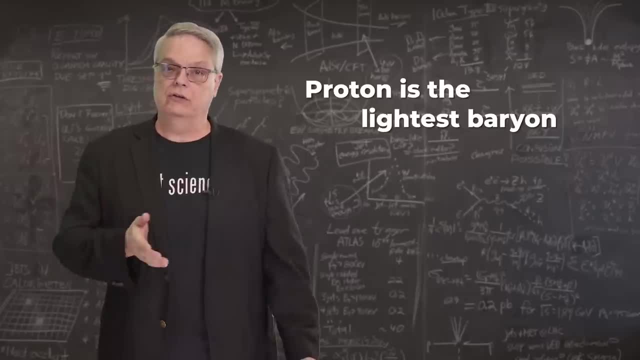 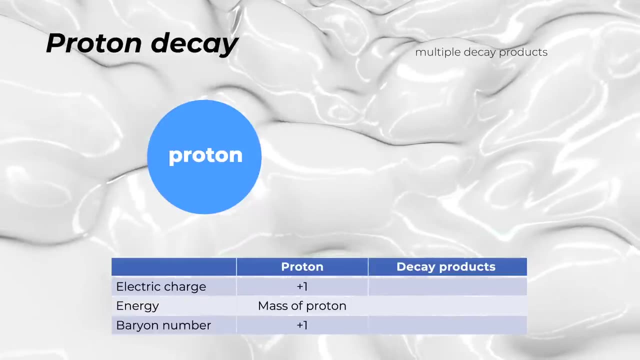 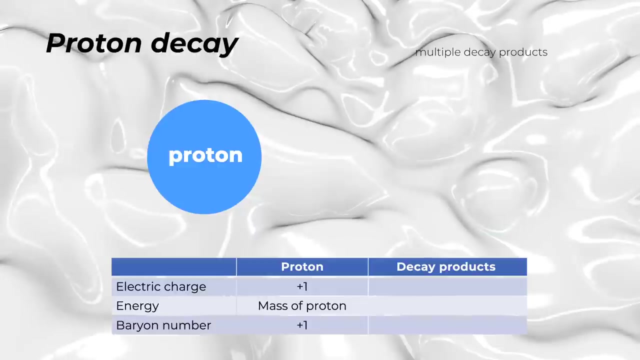 lightest baryon. All other baryons are heavier than the proton. So let's consider proton decay. The standard model says that any decay has to conserve electric charge, energy and baryon number. Thus a proton with a baryon number of plus one and a charge of plus one and a fixed mass. 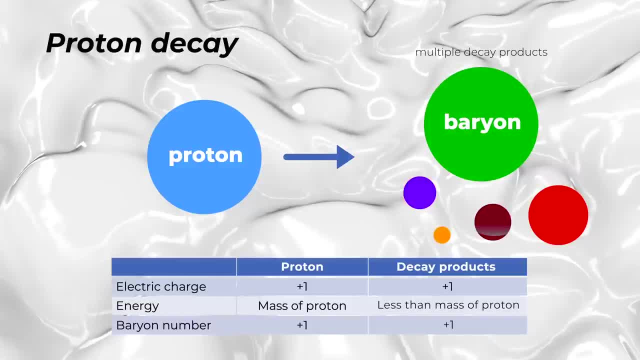 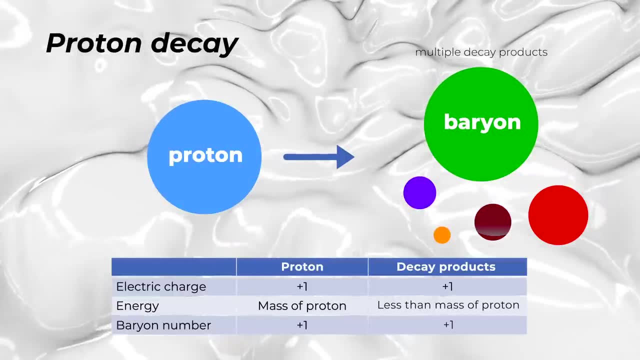 would have to decay into some number of particles that would have to have a total mass less than a proton, a total charge equal to plus one and at least one baryon. But here's the problem: The proton is the lightest baryon. 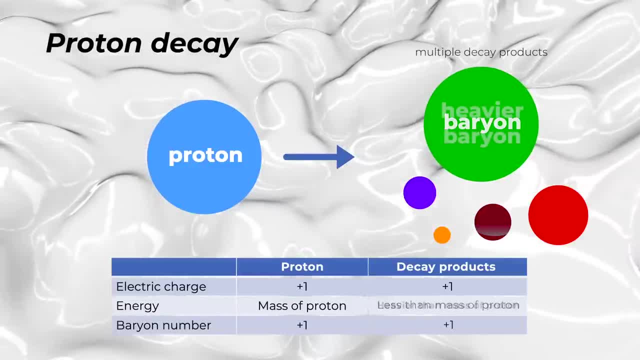 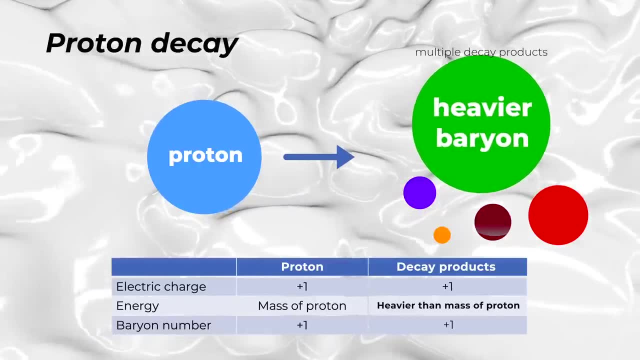 Thus any other baryon is the lightest baryon. Thus any other baryon into which it would decay would be heavier than the proton, And that would violate energy conservation. Therefore, because there is no way for a proton to decay into another baryon of higher mass, 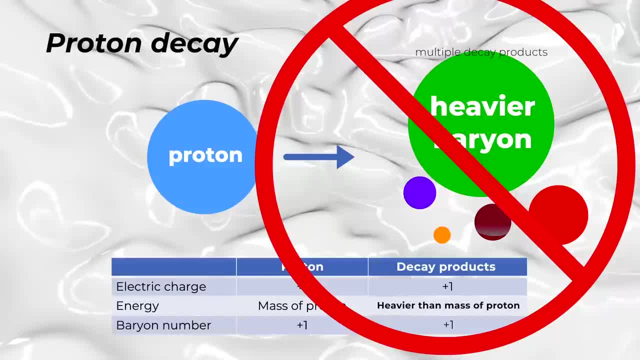 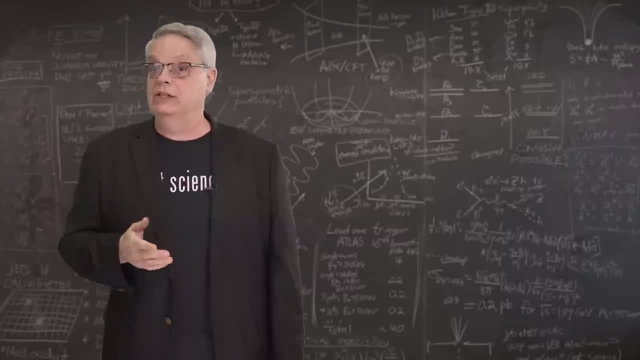 protons can't decay into another baryon And coming full circle. according to the standard model, the proton is therefore stable. That's it The end. However, in some proposed replacements of the standard model, some of those conservation laws are relaxed. 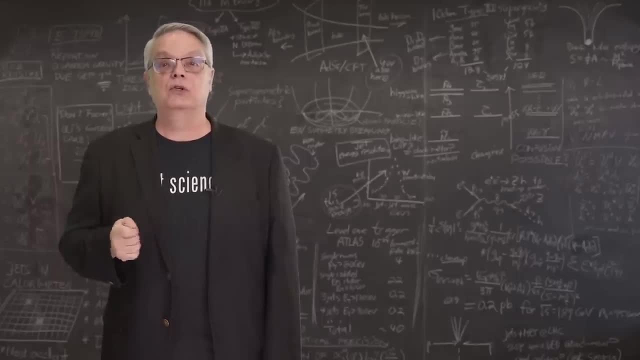 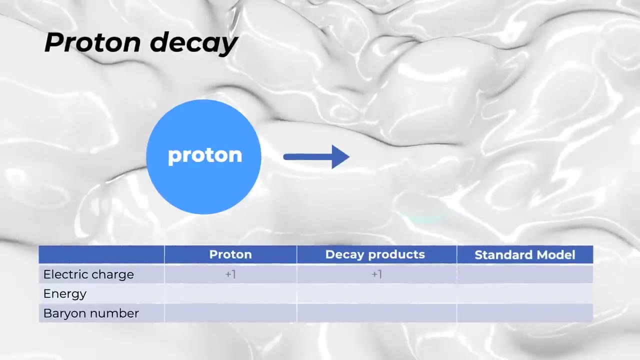 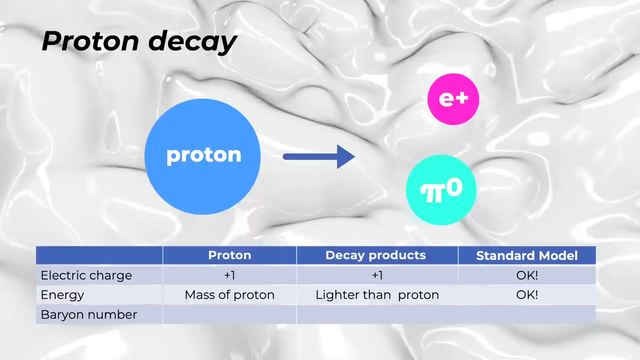 For example, these models often say that a proton could decay into a positron and a pi-maison. We see that in this decay that charge is conserved and the mass of the particles after the decay is smaller than before. so the decay is OK on charge and energy grounds. 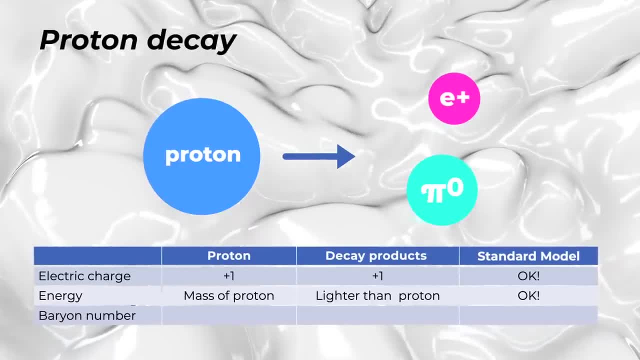 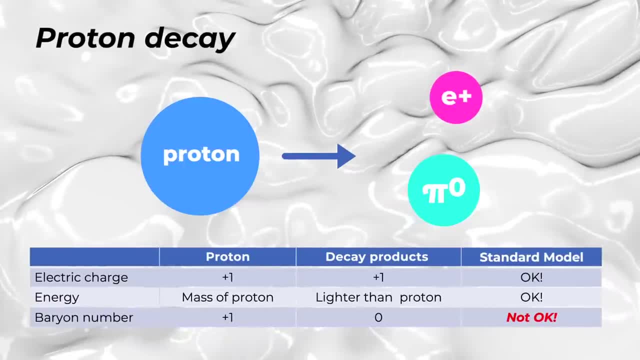 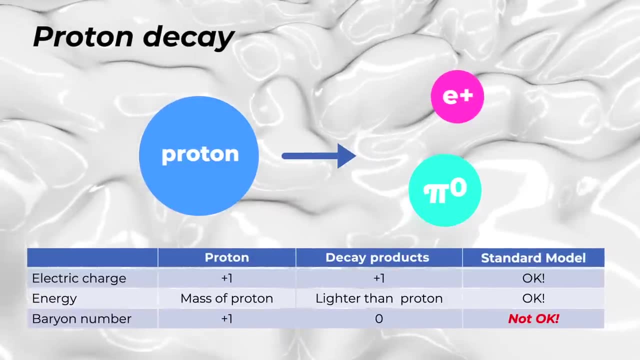 So this decay is forbidden in the standard model, But it's allowed in some possible replacements of the standard model. Thus, observing this decay would be an important validation of new physics theories. On the third hand, we know that protons don't decay very much. 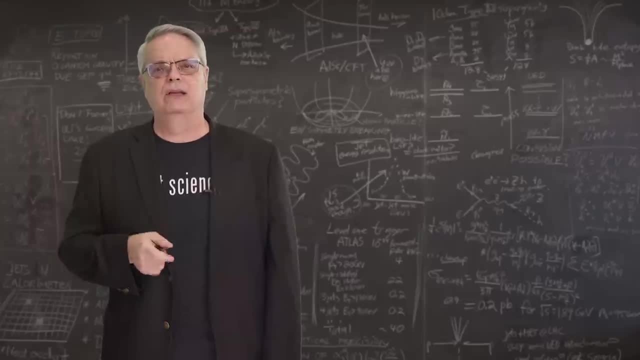 If they did, atoms wouldn't exist and we wouldn't be here. Luckily, these new replacement theories say that the lifetime of the proton is very long. Even back in the 1980s, when these theories were new predictions for the lifetime of 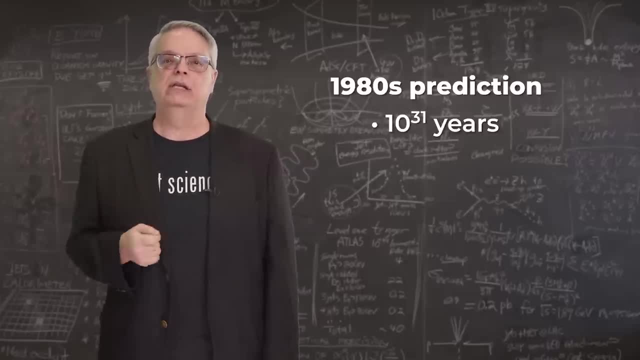 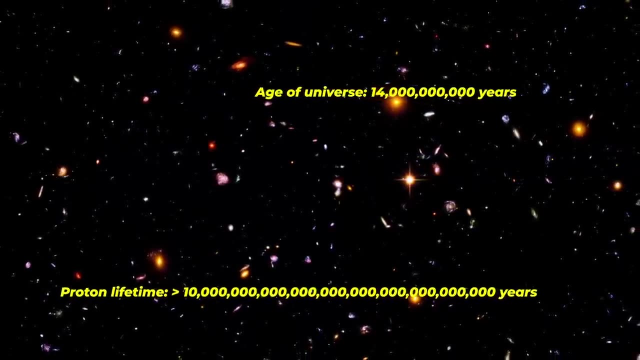 the proton were about 10 to the 31 years. That sounds like a lot, but it's more than that. The universe has been around for 14 billion years. To simplify things, let's call that 10 billion years, or about 10 to the 10th power. 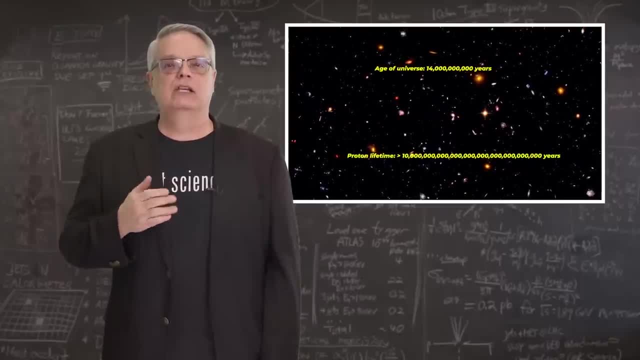 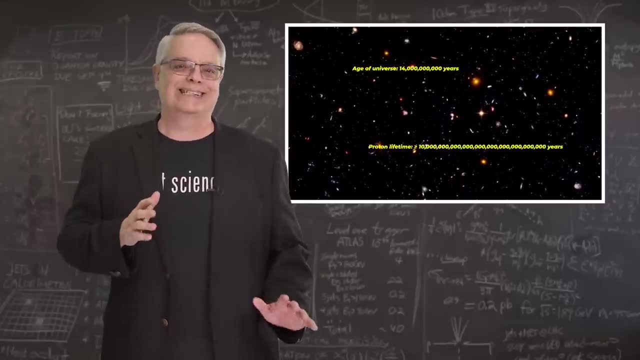 That means that the shortest predicted lifetime of the proton is about 10 to the 21 times longer than the universe has existed. Ten to the 21 is a sextillion. So if you have a single proton, you have a second proton. 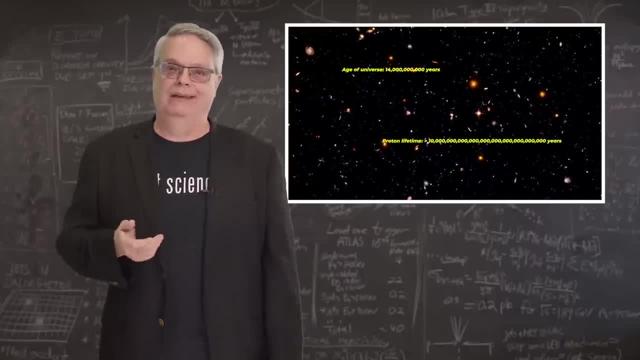 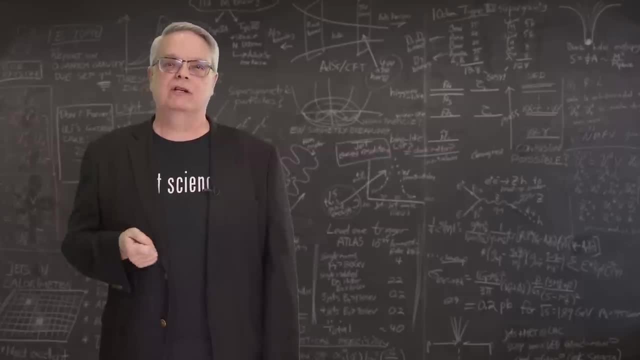 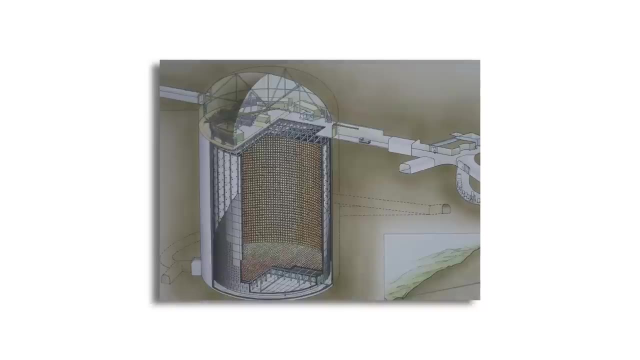 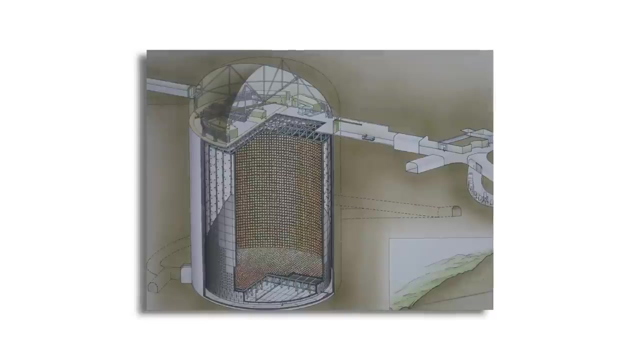 If you do the math, you find that 30,000 metric tons of water contain something like 10 to the 31 power protons. So scientists did just that. They built the Super-K detector, located in Japan. It's a cylindrical tank buried a kilometer underground, or about half a mile. 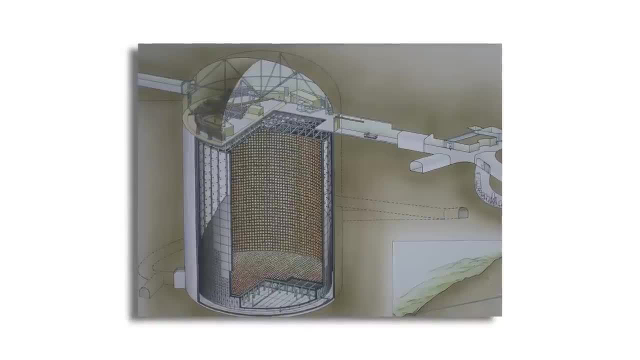 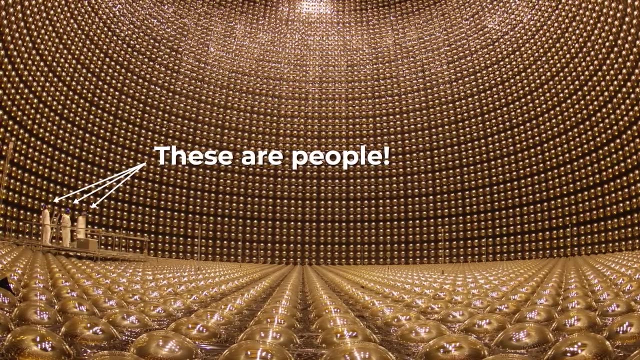 The tank is about 40 meters tall and across, or about 130 feet in both directions, And it's full of ultra-pure water. In 1996, the Super-K scientists turned their detector on and started looking for decaying protons, among other things. 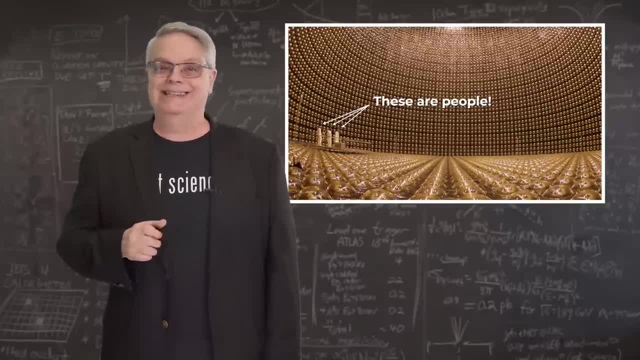 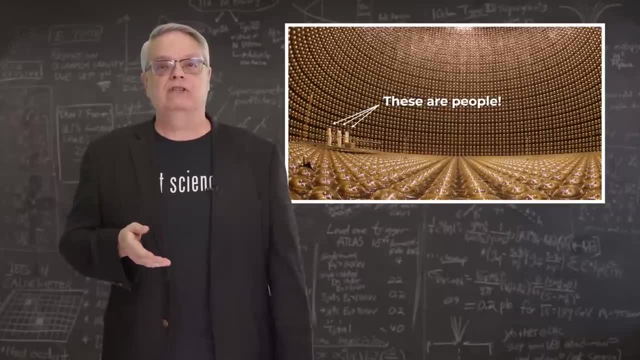 Well, they've made a lot. If they've made a lot of neutrino measurements, they haven't seen a single proton decay From that. researchers have concluded that if protons decay in depositrons, the lifetime for that decay is more than 2 times 10 to the 34 years. So does that mean that protons don't decay? Well, no, we can't say that. All we can say is that they don't decay quickly in depositrons. We need to build bigger detectors to see if protons decay with a lifetime longer than. 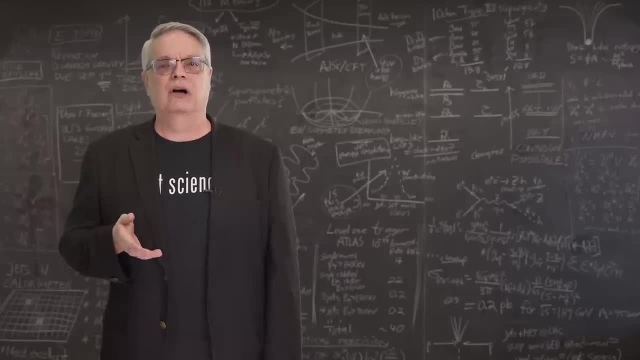 that We also need to build detectors that look for other forms of decay, And at Fermilab we're doing just that. Well, sort of Fermilab is building the Deep Underground Neutrino Experiment, which we call DUNE for. 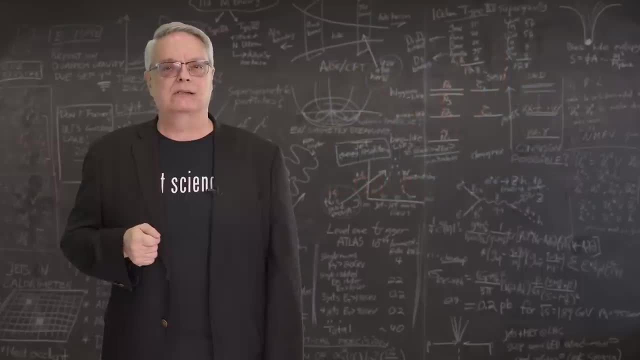 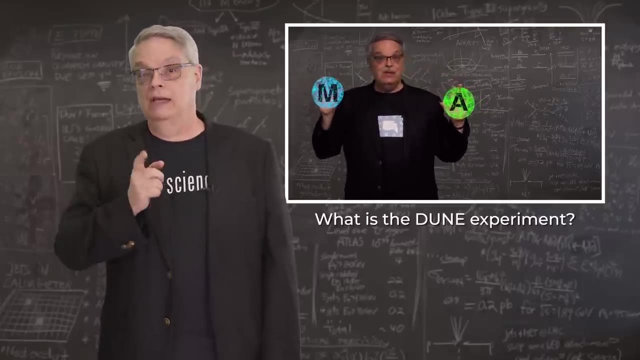 short. The primary reason DUNE is being built is to study the behavior of neutrinos. I made a video about the DUNE experiment. The link is in the video description. However, the DUNE detector will be huge. When completed, it will comprise some 70,000 neutrinos. 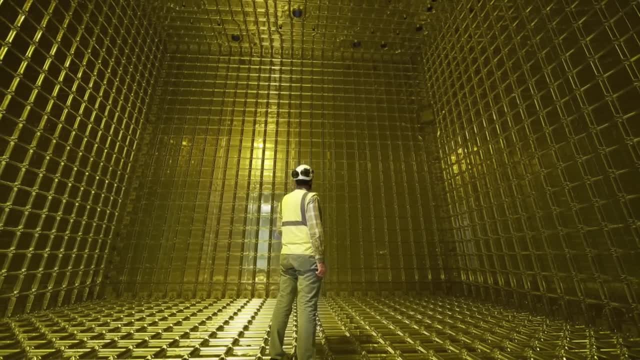 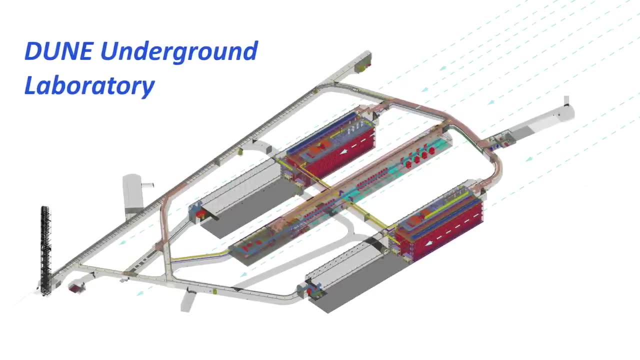 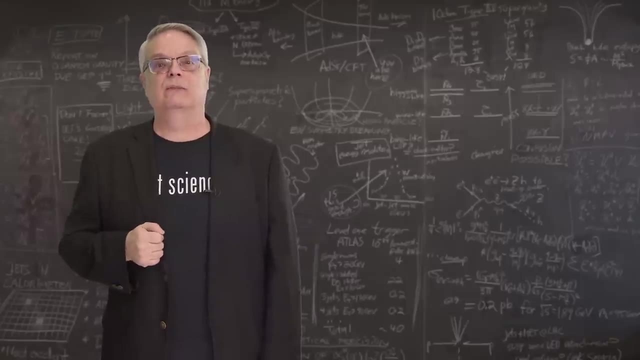 That's a lot. The DUNE detector will consist of over 200,000 tons of liquid argon. While, for technical reasons, not all of that will be available for looking for proton decay, the DUNE detector represents some 20-30,000 tons of useful protons. 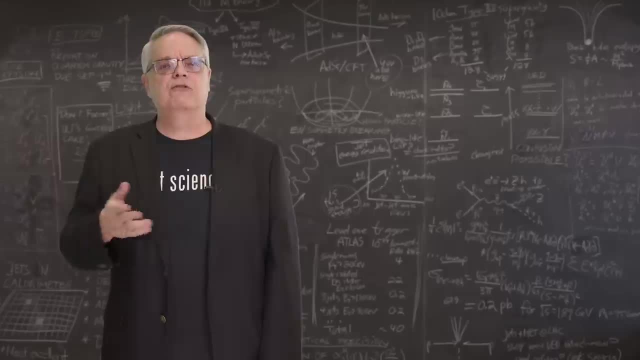 And with all those protons in such a super sensitive detector, scientists will be keeping an eye out for proton decay. There are lots of different theories about how protons will decay, And while the DUNE experiment will be able to see such a decay, the experiment has spectacular 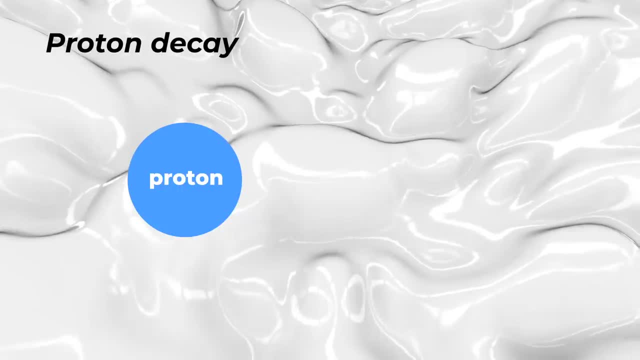 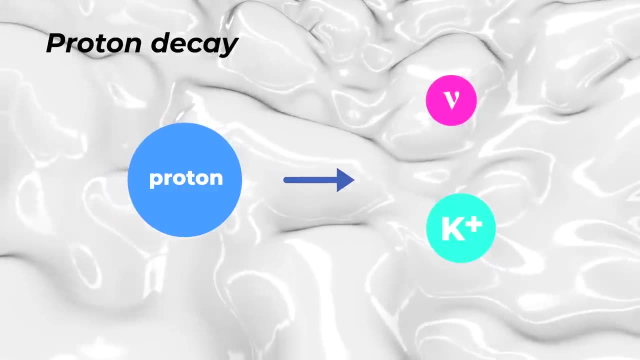 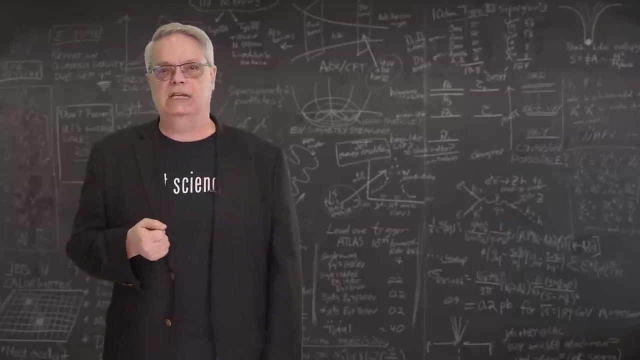 capabilities to look for the possibility that a proton will decay into a positively charged meson along with a neutrino. The DUNE experiment will identify that form of proton decay with excellent efficiency, And that's great news, as the water detectors aren't as sensitive to that particular decay. 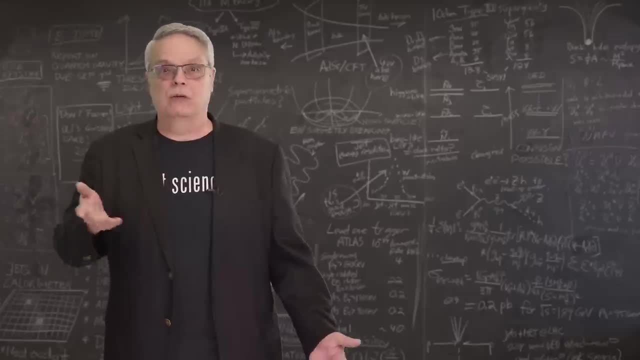 mode. Of course DUNE will also be looking for other possible forms of proton decay as well, But it's the K-meson channel that DUNE dominates. It will be a huge scientific advance if it's seen Long term. it's expected that the DUNE experiment will be twice as sensitive as the competition. 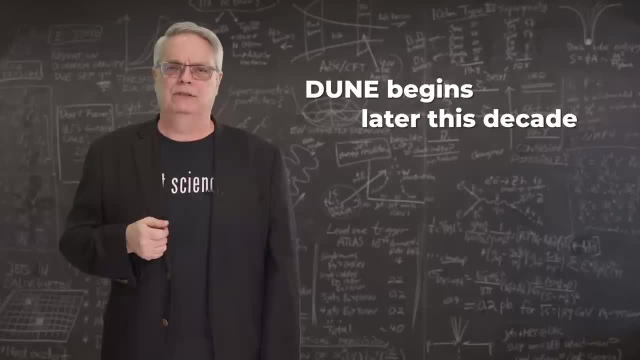 Will DUNE see proton decay? I know how I would bet, but the simple truth is I don't know. That's the thing about research: you don't know the answer until you find it. DUNE is going to be super busy doing neutrino studies. 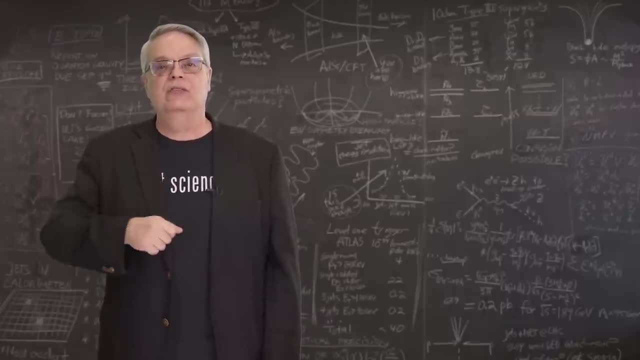 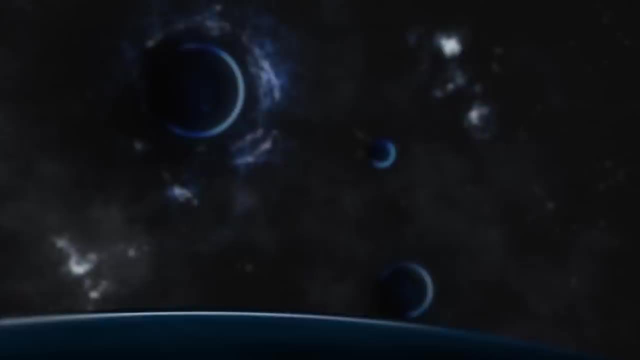 And the proton decay research will be conducted in parallel. Given the implications of seeing proton decay, Fermilab scientists are on it And one day we'll know. OK, so proton decay, if it exists, is a super rare process and one that's very hard to 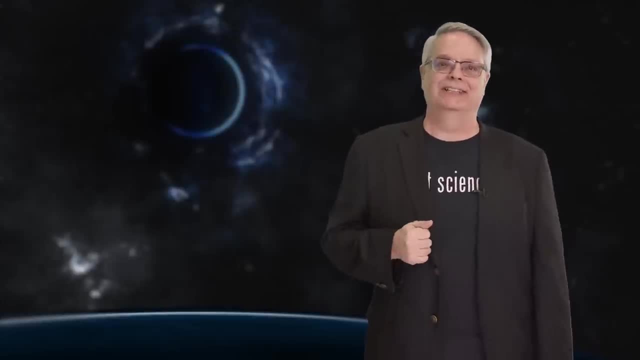 measure, But that's OK. If it were easy, everyone would be doing it. If you like learning about possibly paradigm shifting measurements, please like the video and subscribe to the channel by smashing that button down there. Come on, You want to do it.